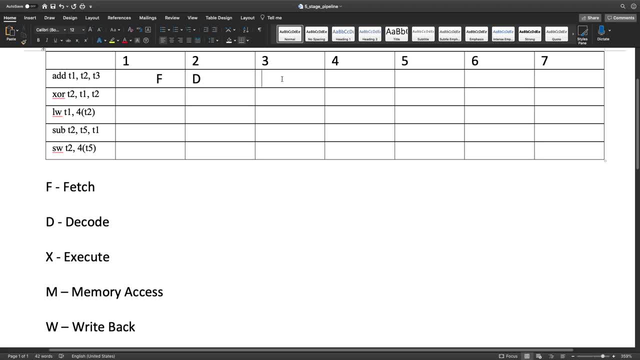 So already we know that, since add is going to the fetch stage, it's going to go without any disruptions: memory access and then write back. and now the interesting part is when we look at the second instruction, as we can see here, we do have a read after write. dependence between the first. 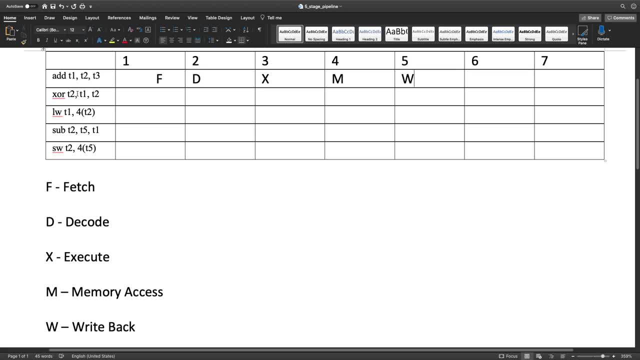 instruction and the second instruction, because the second instruction is utilizing the t1 register, which should have an updated value after this add instruction is executed, but because this dependence can be handled with a, with a bypass operand, we don't. we actually can start the fetching of the second instruction while the add instruction is being decoded, so whenever. 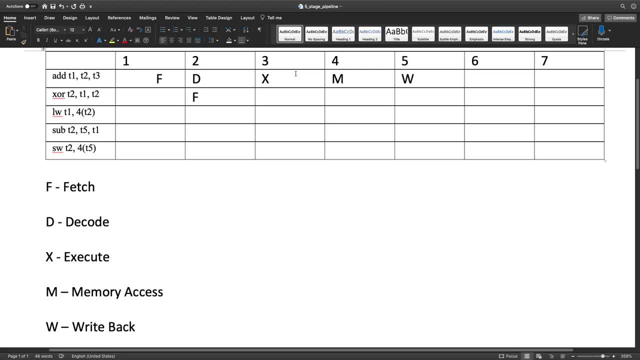 the add instruction is finished executing and t1 has, then we figured out what the new value of t1 is, and then we can start the fetching of the second instruction, and then we can start the fetching of the second instruction, and then we can start the fetching of the second instruction. 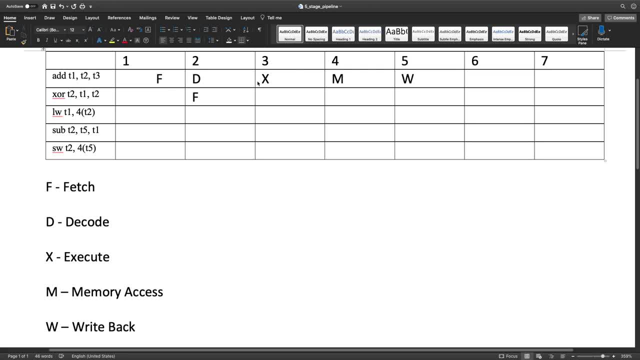 that value is immediately sent or it made available to the in second instruction, so that XOR t2, t1, t2 utilizes the new value of t2 and not the old value, and so we can actually just fill out the cycles right here like normal. and then once again, if we look at the third, 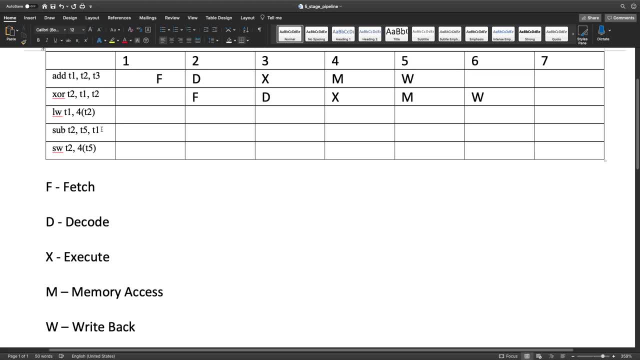 instruction: load word t1 for t2. this instruction is using the t1 and t2 registers and the t2 register's value will change after the previous xor operation but once again, because of forwarding or bypassing, that value is made available almost immediately to to this current third instruction, so we don't have to worry. 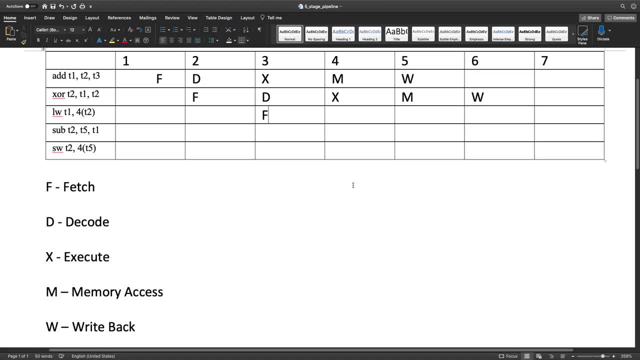 about delaying our pipeline, so we can just start the fetch of this instruction during the decode of the previous instruction and then go on as usual with decode, execute, memory access, right back. and now this next instruction is where we run into some issues, as you can see. again there's 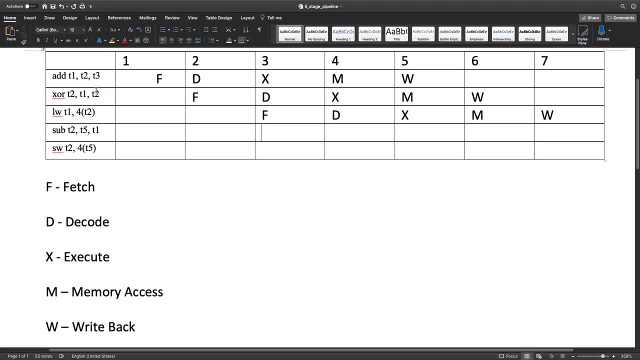 a read after write. dependence here because sub t2, t5, t1 is utilizing the t1 register and it wants to get that value and t1 is being filled in with whatever value is at the four, four byte offset from t2 in memory, but because load word involves memory access. so 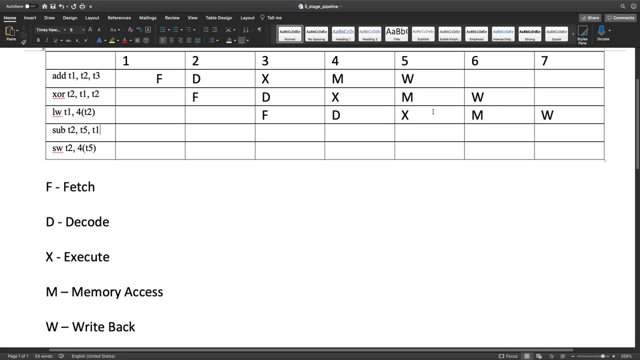 accessing data from memory. we're not able to forward or bypass that that result immediately to the sub instruction. so we actually have to wait until this instruction is properly executed, that and the memory is accessed and that result is written back into the t1 register. so what we do is we can still. we can still fetch the instruction, while the previous instruction 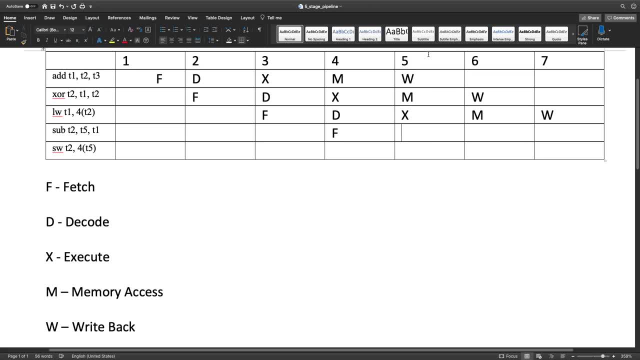 is being decoded, but in the fifth cycle we actually have to delay that and we can't start decoding or executing until we skip that one cycle. because by skipping that one cycle we're able to guarantee we're getting some Cons viewer into the back row and then webay them in the back row. and then we back up this same instruction using the same slash key palm and just say: I'm out of the HFSiva package, which actually allows you to use that flag in the army. cikk whenever there's a new application slip that you can just type it in that ingunit or anything that needs to be done. so we might just and cikk any of therietlicy. we might have to actually figure out if there walls to string them in some way. so if the wall is planet, we want to have that one off for. 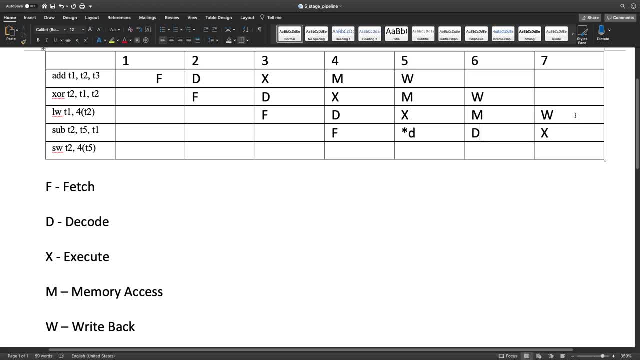 that the memory is. we have to wait for the memory to be accessed and for the results be written back before we can execute this instruction and then the next instruction. actually, we can go as normal it's. it's it's only using the t2 and t5 registers, which there's no read after write dependence. here we're. 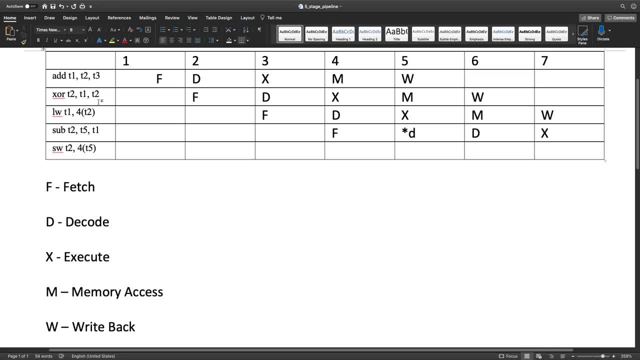 reading from t5. but t5 was never written to previously and in this case we can just start with the fetch on the fetch in cycle 6 while the sub instructions being decoded, and then decode this one right here and notice that I didn't put the fetch of this last instruction in cycle 5, because when we 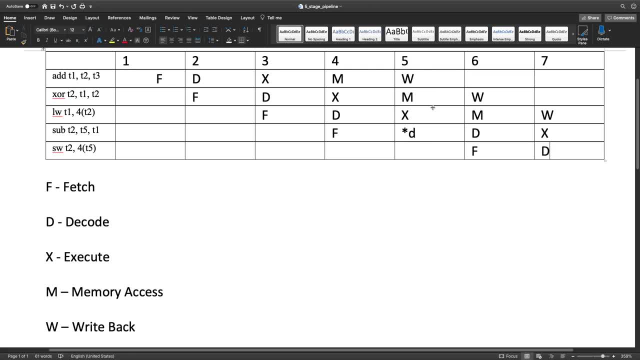 delay the pipeline, we're delaying the, essentially delaying the entire circuit or the entire processor. so we're not able to perform anything while while this delay is happening.